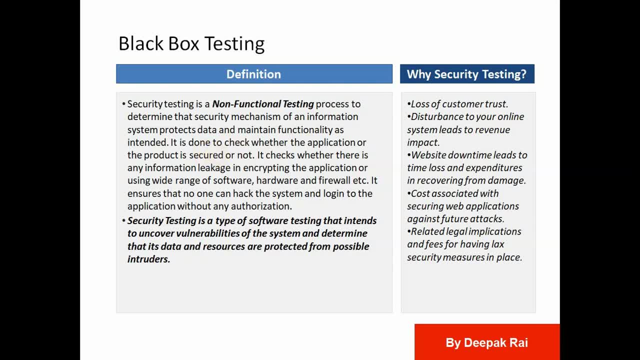 It means it's a part of functionality testing which we are using for securing the data and their other stuff from the viruses or from the attackers. It is done to check whether the application or the product is secured or not. It checks whether there is any information leakage in encrypting the application or using wide range of software, hardware and firewalls, So, etc. So whenever you're using any application or you, sometimes you- you can get the 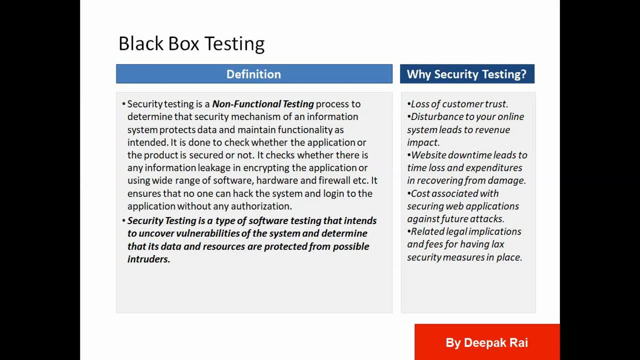 pop-up of your firewall is blocking that pop-up, So it is intended to make your application is secured. and firewall, because that firewall is blocking any unrestricted resources or unrestricted access to your system. So because of that, sometimes we are receiving pop-ups or whenever we are opening any browser, So the some of the times the pop-up is blocked from the browser. So it's intended to make your application secure. and firewall, because that firewall is blocking any unrestricted resources or unrestricted access to your system. So because of that, sometimes we are receiving pop-ups or whenever we are opening any browser, So the some of the times the pop-up is blocked from the browser. So it's intended to make your application secure. and firewall, because that firewall is blocking any unrestricted resources or unrestricted access to your system. So because of that, sometimes we are receiving pop-ups or whenever we are opening any browser, So it's intended to make your application secure. and firewall, because that firewall is blocking any unrestricted resources or unrestricted. 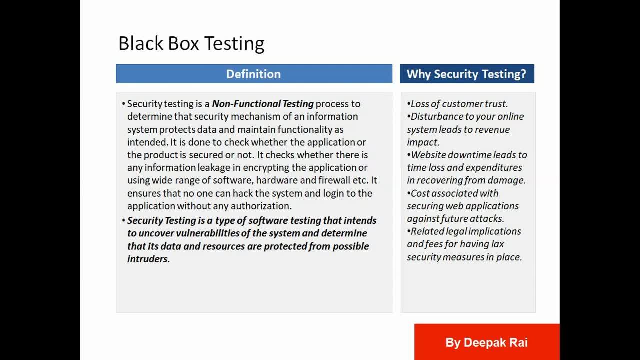 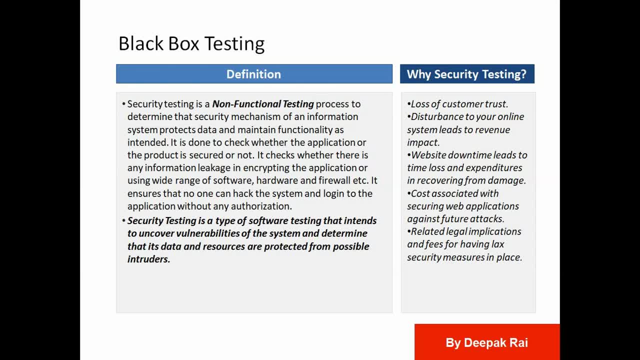 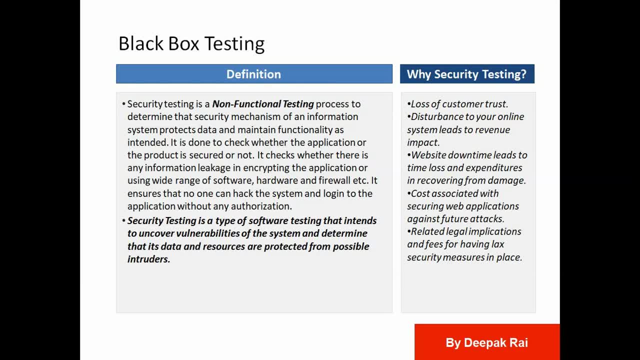 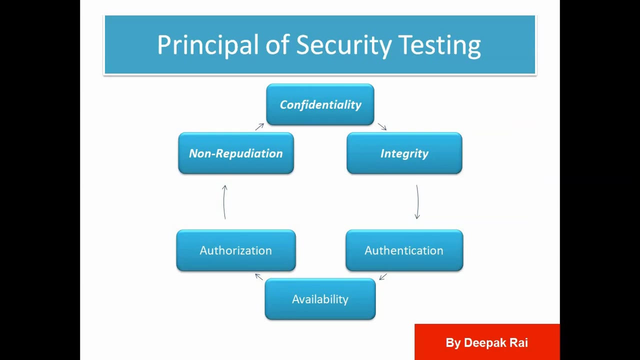 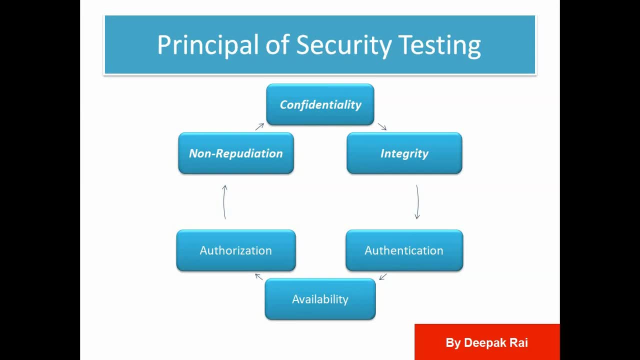 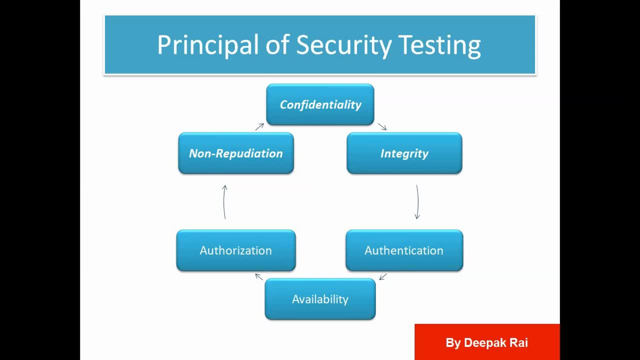 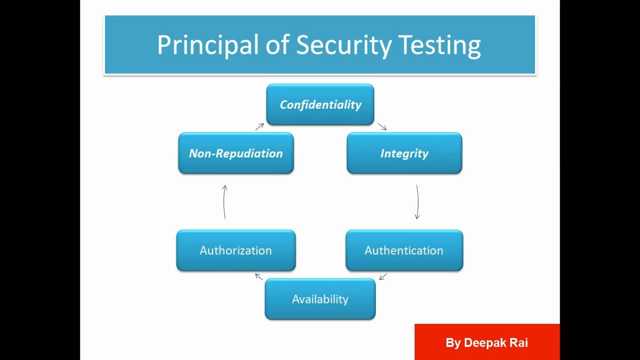 same netbank application and that is authenticated to myself. only availability. it is available for the authenticated user. that is called as availability. authorization authorized to the proper user is called as authorization, like if there are two softwares- or you can call as applications are allowed to download. each and everyone with the authorization code or you can. 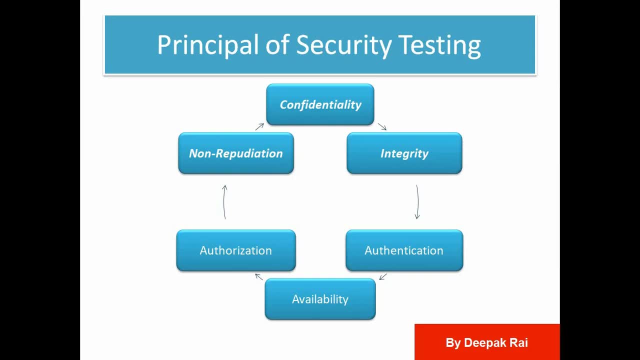 what race in login, like if I am trying to download Facebook messenger. so it is a while for everyone. but it is authorized to use for the by using their username and password. non reputation means non repeating, contained or redundant data to be entered into our environment. so there's. 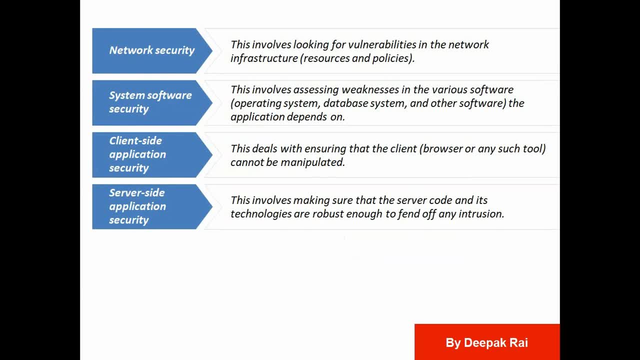 four types of security testing focus area considered in security testing. so firstly, networks are network security. network security is very important part, like if you are working with the MNC company or multinational organization so that organization or network should be secured. like if I am using myself or my router connection so that nectar should be secured for are trying. 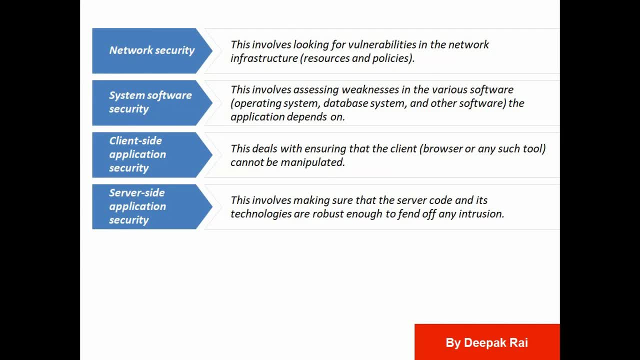 to log in in any of the private data. you can called as net banking login or you can call as any personal application, social media application as well. so network security is very important part in uh. if this involves looking for vulnerabilities in the network infrastructure. that is called as resources and policies. so resources and policies. 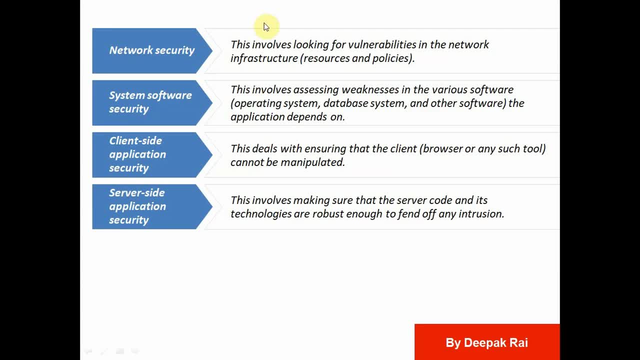 already defined in cyber crime as well. so that will make a major differences for the network. network security system. software security: this is null. involves assessing weakness in the various software, operating system, database system and other software that application depends on the system. software security: client side application security: this deals with ensuring that the client 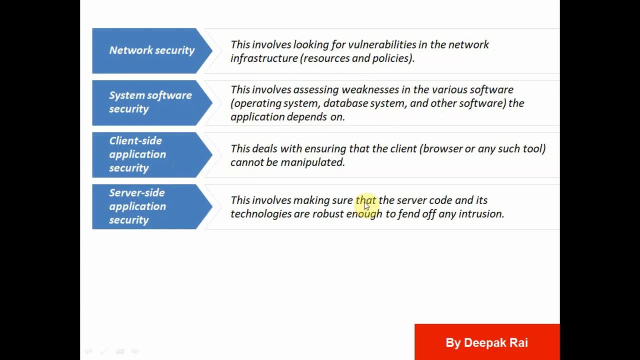 browser. any such tool cannot be manipulated. like if i am using any application, that application should not be manipulated. like there are various application duplicate application available for the whatsapp as well. so for those who is using duplicate application of offset whatsapp that they might come into the network, secure application security or they they have or they can be paid for that. 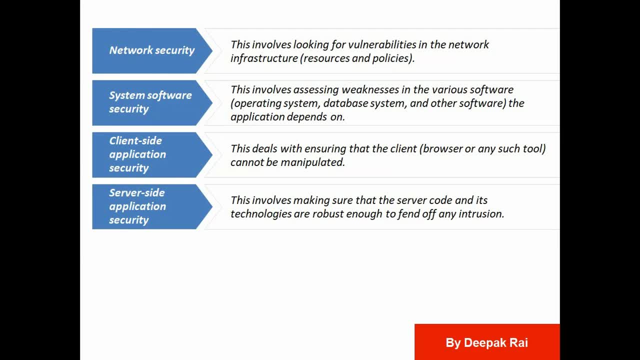 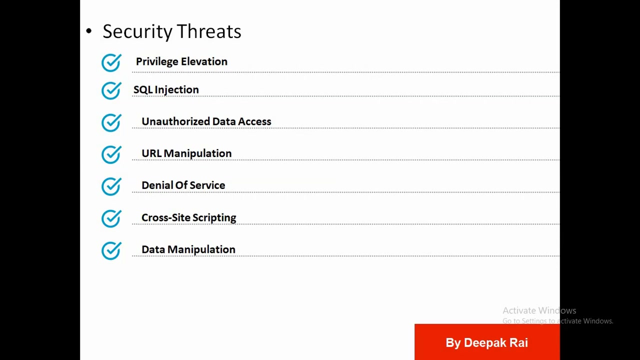 so might be. the hackers will attack on their system- and hackers are not the system- and they can make a theft of any important data. server side application security: this involves making sure that a server code and its technologies are robust enough to stand off any intrusion. so there are total seven security threats. that is first is priveless. 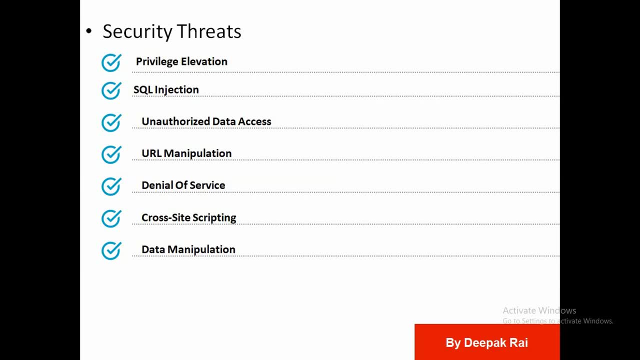 innovation. second is sql injection. third is unauthorized datasaver: 5c2 tests and voltage swinging checks to improveおい ChineSO wissenerm ע. wir sind noch Doub sortir Ид há Upper lid data access. fourth is URL manipulation: your man vision, basically like if I am. 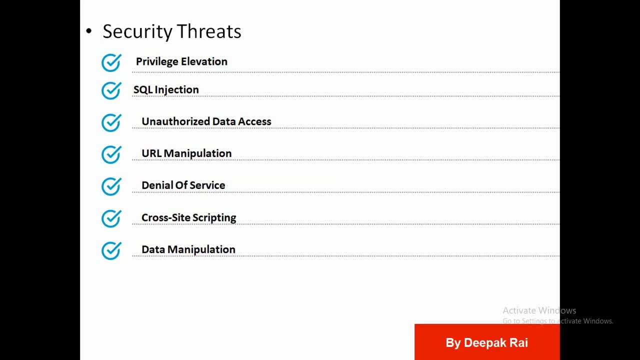 using googlecom and someone is trying to make a scene application with the small changes like Google's dot-com, or you can call as G o L. the name is Google G double o L e, so without placing last e, they can only make G o o l dot-com. so 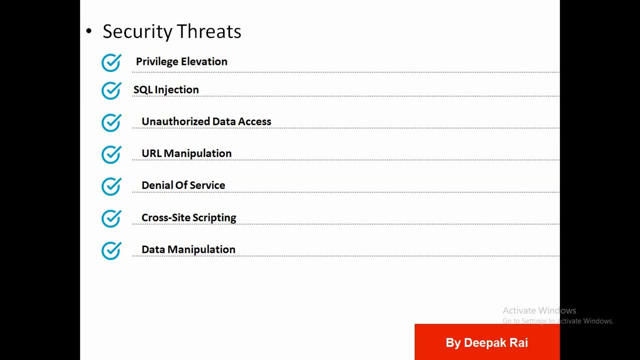 that is called, as you are manipulation, unauthorized data access, so my private data is secured for me and if someone else trying to access that data, it is called as an authorized data access. or, in terms of example, if my company website or they have stored some data in their database and for those who who would. 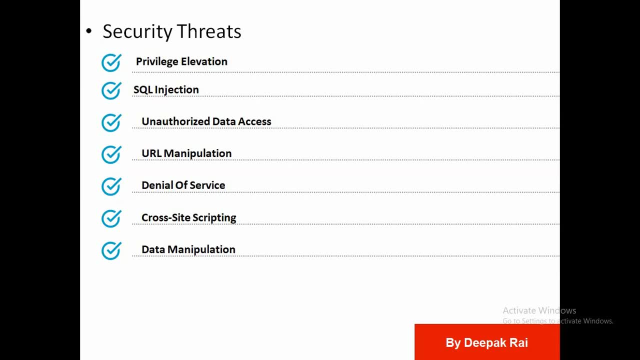 is not authorized to that data and they are trying to access that data is called as unauthorized data access venue of service. then the sixth one is cross-site scripting, that is called as x-axis. and seventh is the seventh one is data manipulation: changing in the name of data. that is all about the security threats. 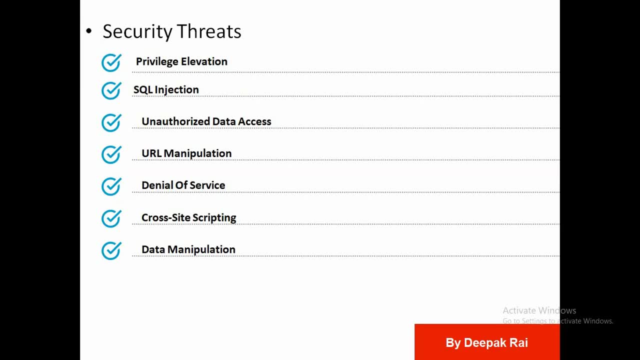 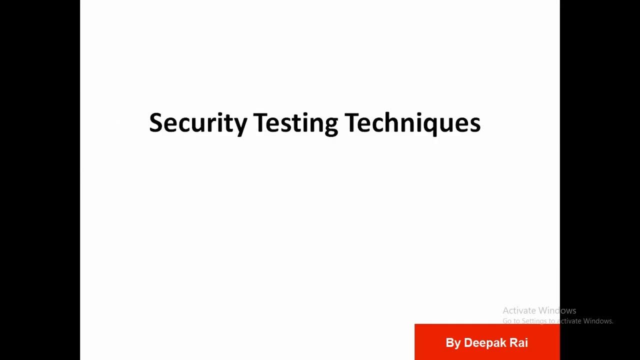 so there is a security testing techniques available as well. first is sql injection, and the sql injection is- entering a single code in any text box- should be rejected by the application instead of if the tester encounters a database error, it means that the user input is inserted in some query and that is executed by the application. so this is all about the sql. 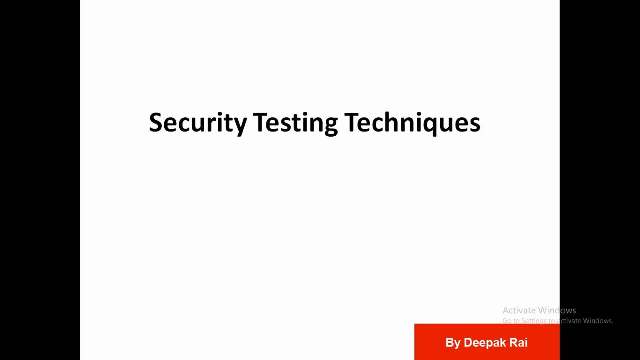 injection. second one is cross-site scripting, that is, x-axis. the tester should additionally check the web application for x-axis cross side scripting. Any HTML example HTML or any script script should not be accepted by the application. Ethical hacking. This helps to identify potential threats on a computer or 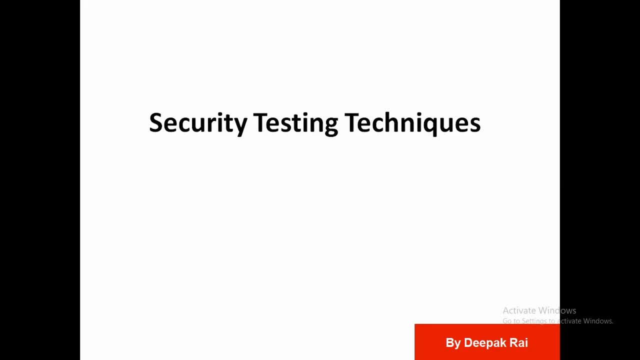 network, An ethical hacker attempts to bypass the system security and search for any vulnerability that could be exploited by malicious hacker, aka black hats. Fourth is password cracking, So guessing the passwords. or if you are trying to log in your private application or private data or private social media network and someone is standing behind you and they are watching your. 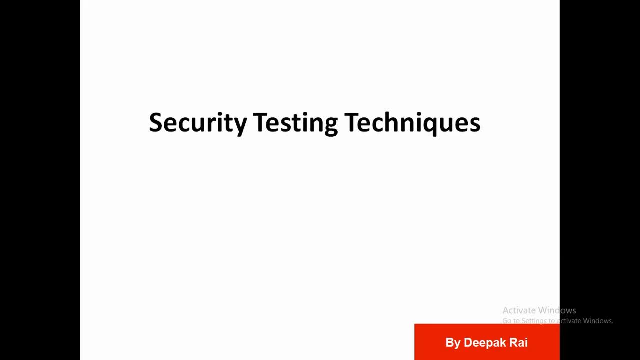 password, so that is also comes under the password cracking. Hackers can use a password cracking tools to crack password until a web application enforces a complex password, Long password with combination of numbers, letters and special characters. There are various hacking applications also available for the password cracking and that. 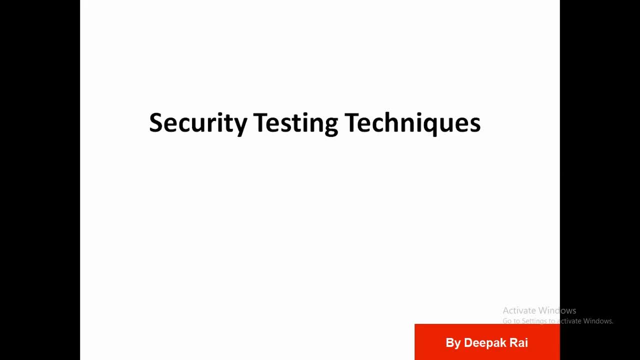 password cracking should be used for hacking your content or making changes in your personal data. Penetration testing: A penetration test is an attack on a computer system with the intention of finding security loopholes, potential gaining access to it, its functionality and data. Risk assessment: This is a process of assessing and deciding on the risk involved with the type of 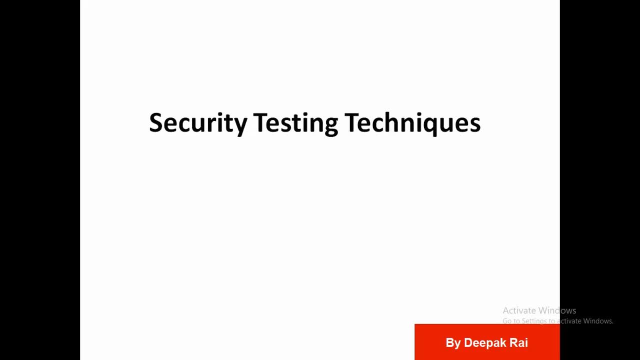 loss and the possibility of vulnerability occurrence. Security auditing: A security audit is a systematic evaluation of the security of a company's information system by measuring how well it conforms to set established criteria. Security scanning: This is a program which communicates with the web application through the web front-end in order to identify